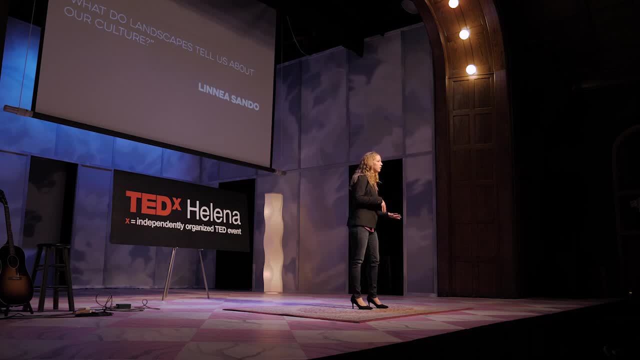 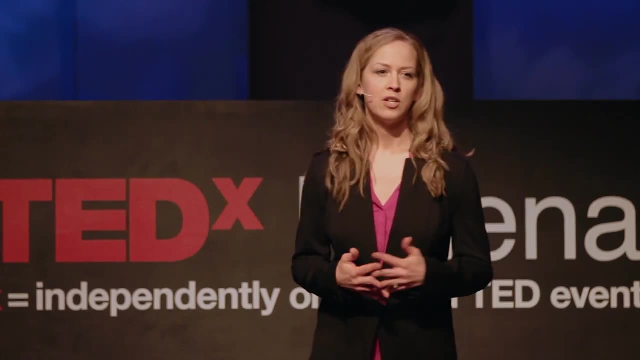 Well, one: we live in it. The big box stores, the small locally owned stores, the suburbs, the sidewalks, the streets are all part of the landscape and guide us in our day-to-day living. Two: simply a deeper appreciation for places and the processes that go into creating those places, the people who are. 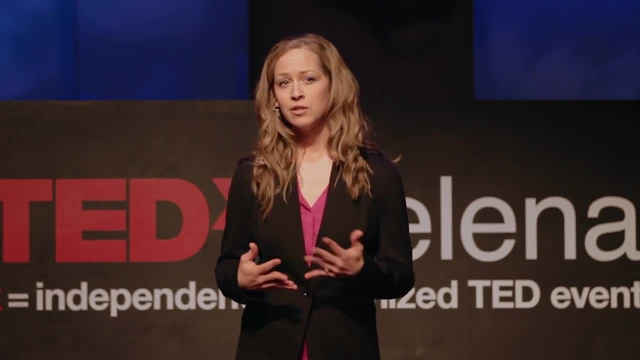 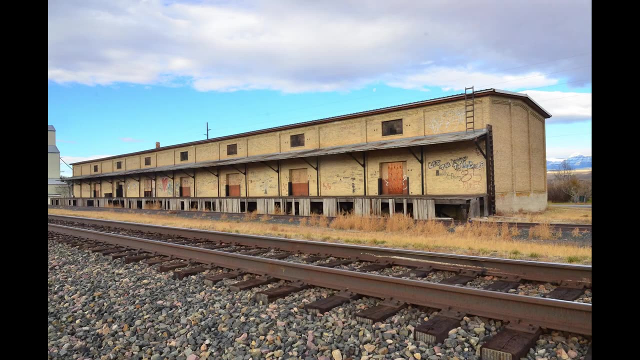 involved, the labor that's involved, And then knowing that there are individual and community stories that surround each and every landscape. So if we take a look at this building here, the Wool Warehouse- this is in Big Timber, Montana, And it might not look like much of a building. 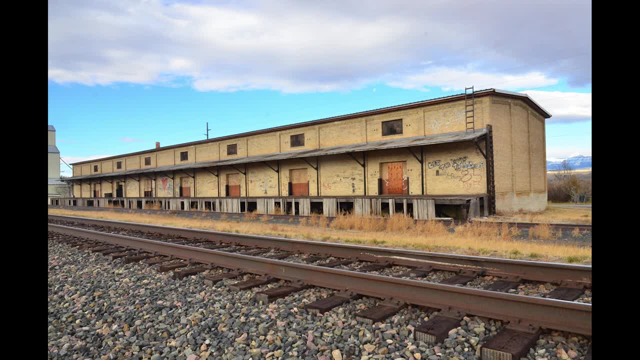 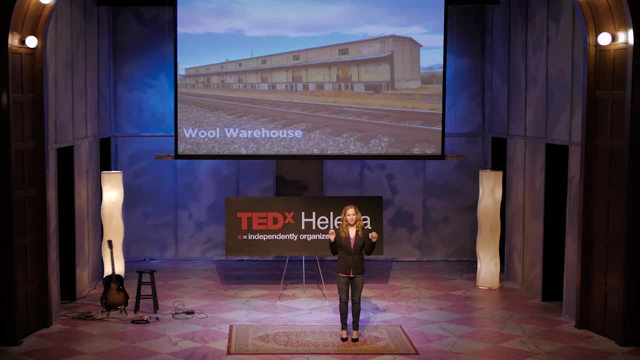 but it stands as a reflection of the community's heritage in Big Timber and that it was its historical foundation with the sheep industry. And the really neat thing is if you step inside that building and it's brick walls all around and what you'll see? you'll see dates and signatures, some over a hundred years. 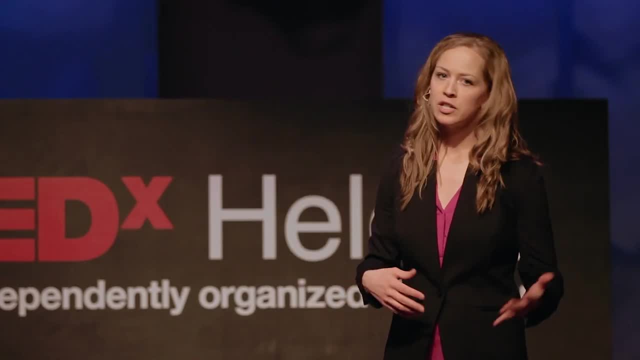 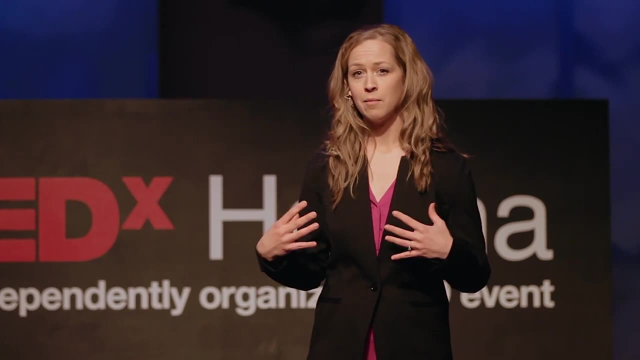 old, from anybody who had anything to do with the industry, whether they're wool stompers, shears, herders, ranchers. And so you have this building that's a reflection of the community's heritage in the industry, but then, attached to that building, you have individual stories of family. 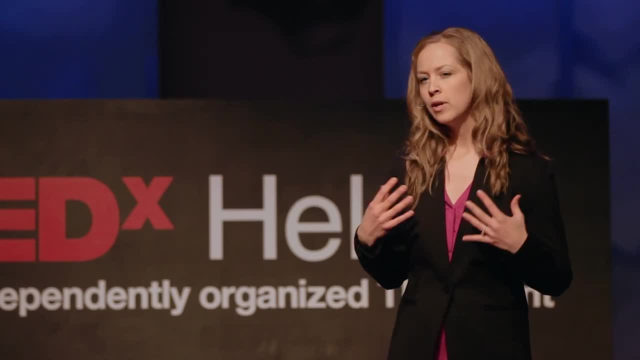 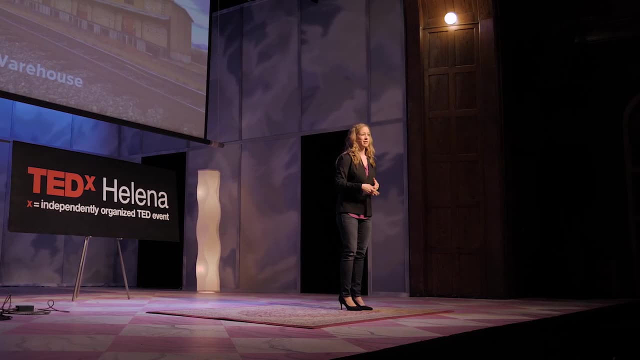 of friendship, of labor and of that hard work. And so when we know more about the landscape and the meanings behind them, we tend to take better care of them and we appreciate them more. And so, whether that's a building that makes your community unique, or, say, public lands that surround your, 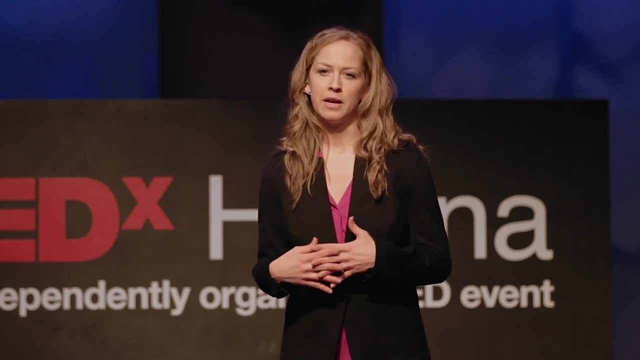 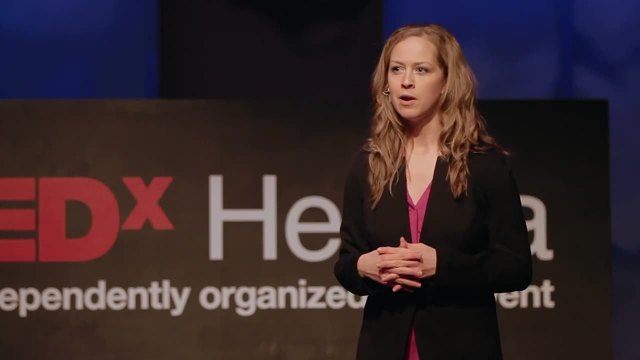 community. So what else can we learn from the landscape? What can we look for? Well, we can learn about the past. We can learn about you know who people are, where they came from, And so one way to do that is look at ethnic signatures on the landscape and ask the question: why? So? why did a 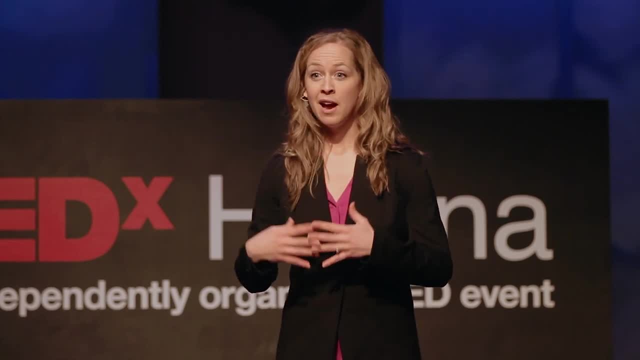 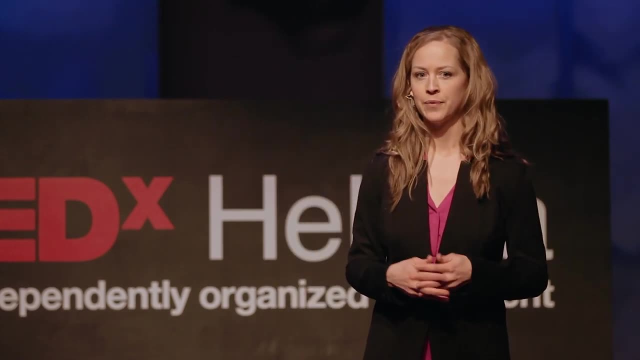 particular group of people settle in a particular landscape And then, in turn, how did they shape that landscape and how did the traditions that they brought with them? how is it continuing to shape that place- identity- today? So an example of this would be if we go to Elko Nevada. 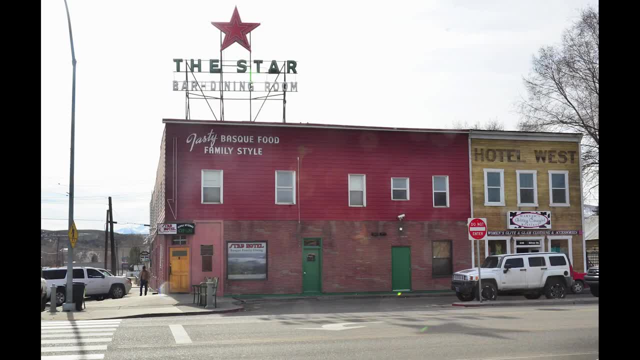 northeastern Nevada and we have the Star Hotel here. You can see it says Basque food. And going back to the why, why did the Basques from France and Spain come to Elko Nevada? And that goes back to the sheep industry also. They came in the late 1800s, first half of the 1900s, to work as herders. 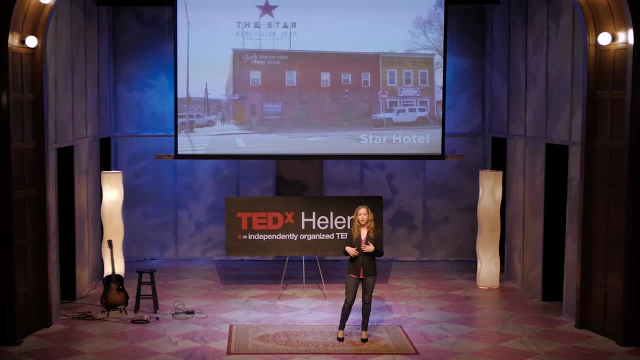 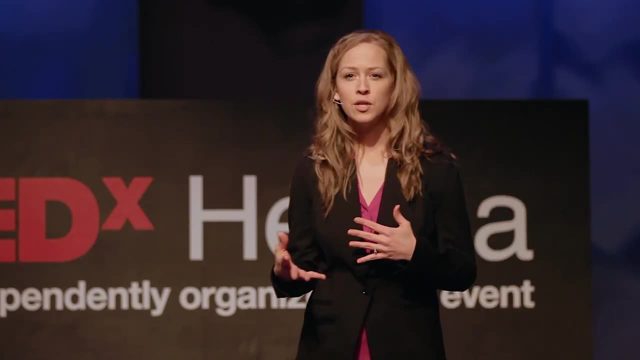 And then other Basques came and they built these Basque boarding houses, which is a combination of a restaurant and a hotel, And they were used to accommodate the herders and provided them a home away from home where their languages were spoken, customs and traditions could be carried on, And today this 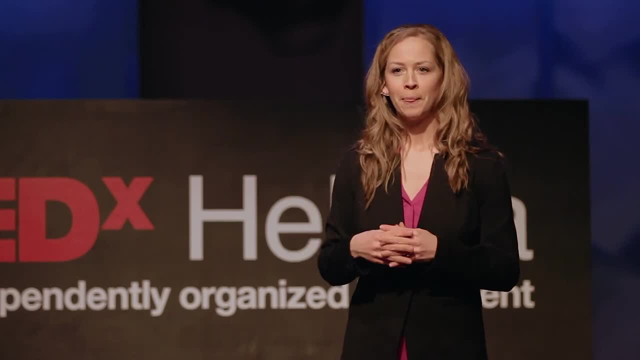 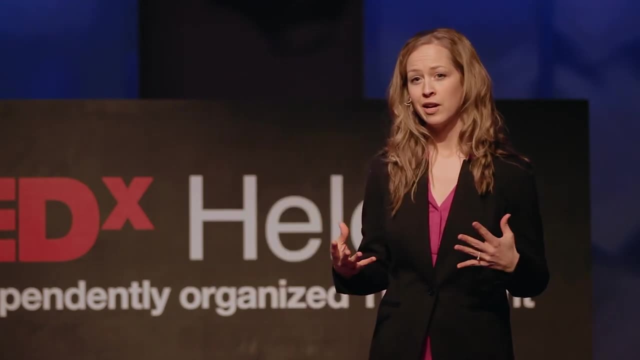 one, the Star Hotel, built in 1910, remains. And so, although you know it's not a boarding house or it's not a hotel anymore, it is still a restaurant, And those traditions, then, are still carried on within those walls and also within the greater Elko community. And so, when we have 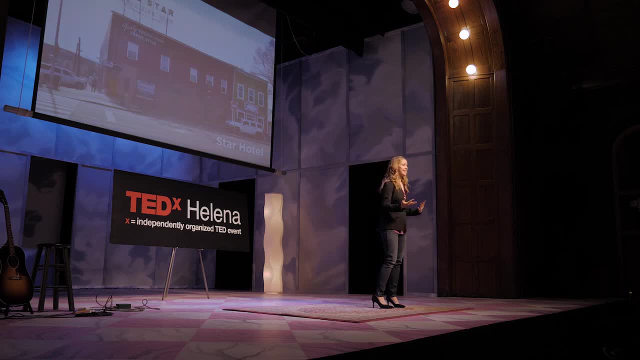 these ethnic signatures, whether it is a restaurant or, say, Finnish saunas, on the landscape is a reminder of the culture's heritage, And although that heritage might be reimagined in slight or big ways, it's still a connection to the past and showing that traditions are carried. 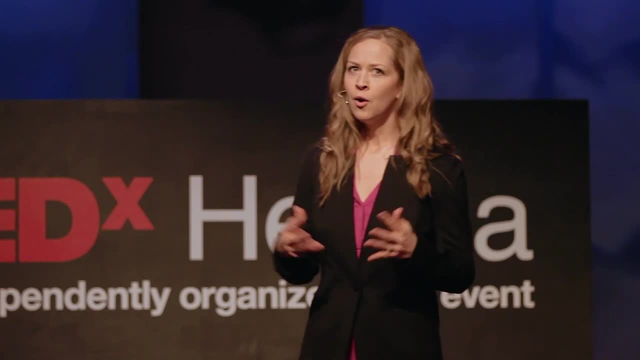 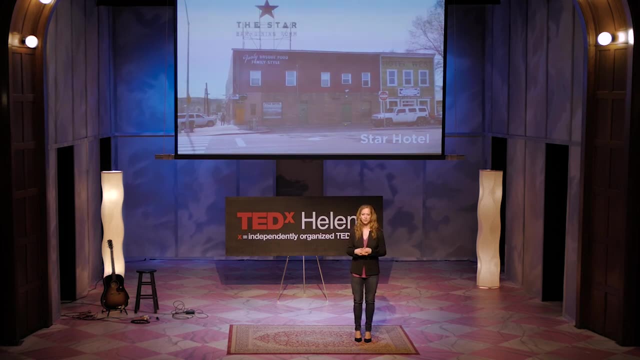 on and it still shapes those places. then today, What else can we learn? We can learn about how culture has evolved and how it's changed. And so if we just meander west of here towards, say, the Avon area- and I'm sure many of you have driven that road before you've, maybe even 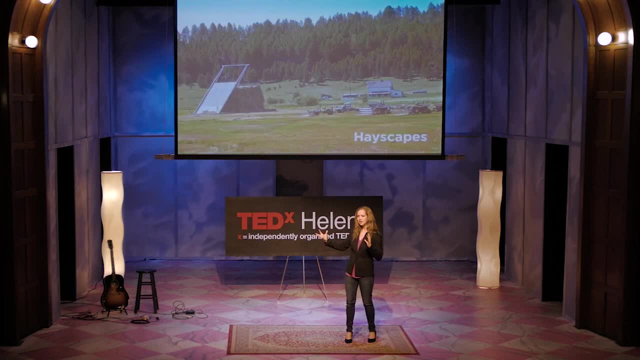 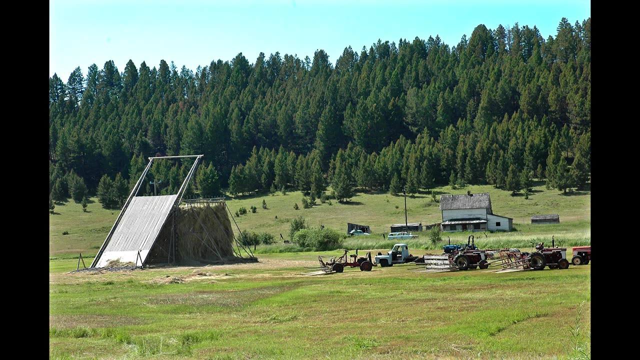 seen these type of landscapes, with the big, huge haystacks right and the strange contraptions that are next to them, And they're picturesque, to be sure, but they also tell us how culture has evolved, how the scale of ranching and farming has evolved, how families and labor 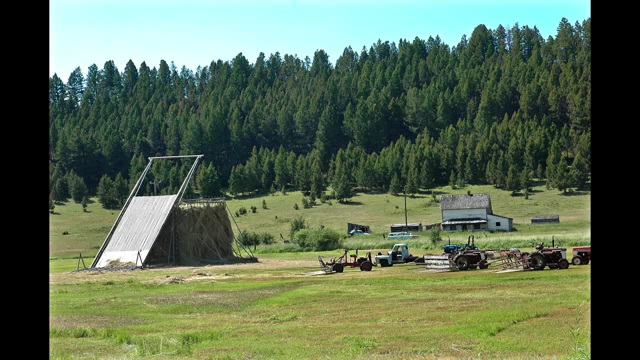 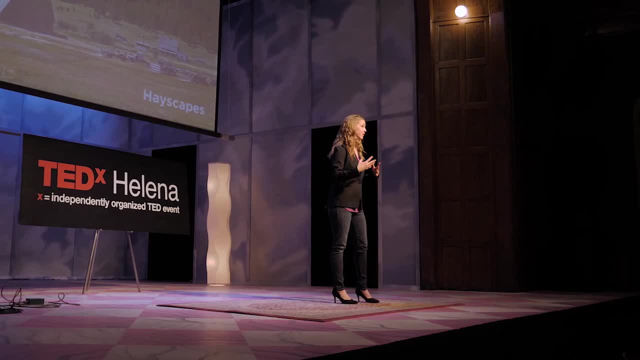 have changed. So this used to be a common way to put up hay, but it was also very labor-intensive. It took a lot of people, which wasn't always necessarily a problem. Families were larger, so you could find the labor pool within your own family, within the community, even itinerant. 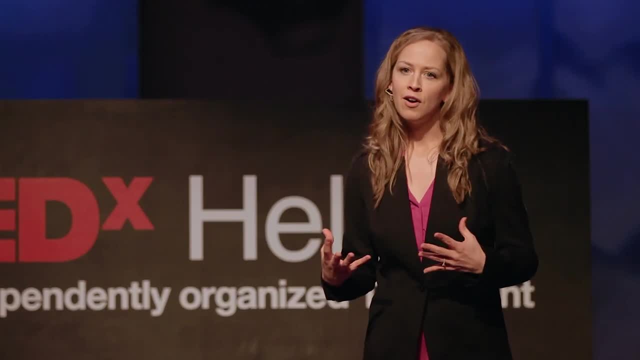 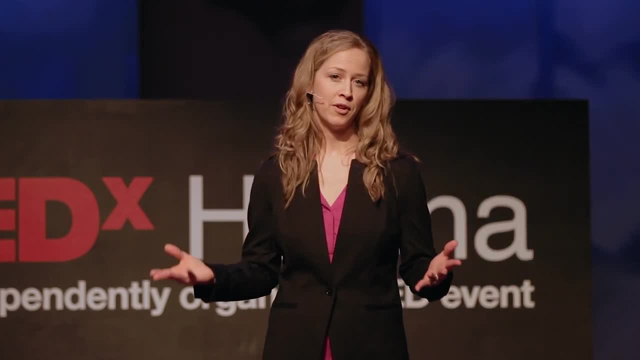 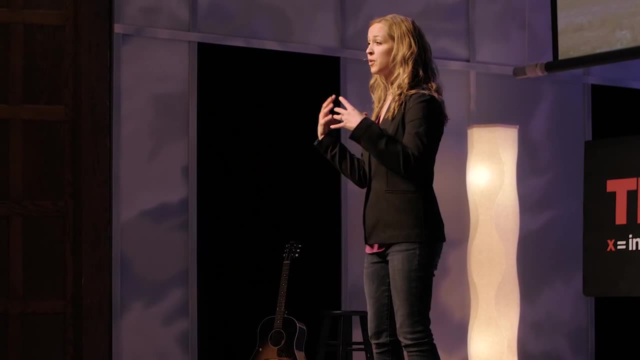 so families are smaller and now you can just have one or two people and a tractor and hay baler put up your hay, And so we can think of our landscape as layers. Right, There's going to be aspects of the past, but then there's also the present and our contemporary. 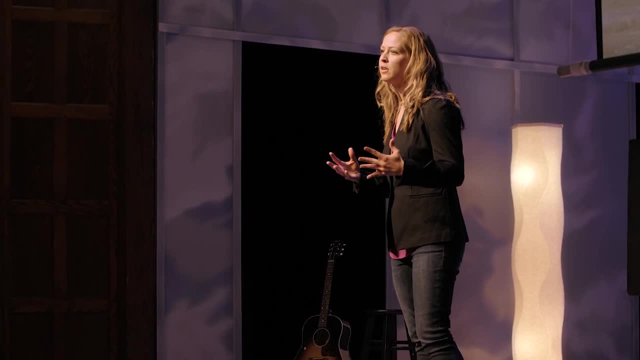 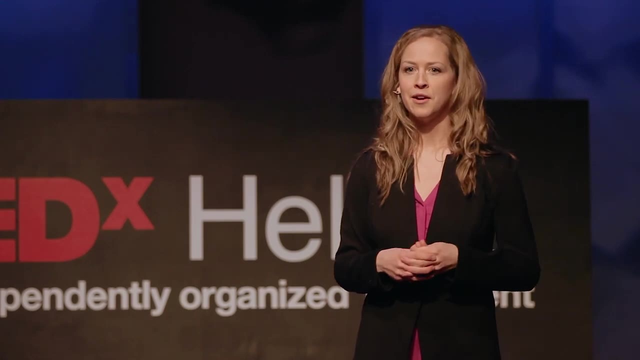 values. So what do we value? How is that different from community to community? and how does that? how is that reflected on the landscape? So let's take a look at a local example. Here in Helena, we have our trails right And you have your signs: Mount Helena City Park. 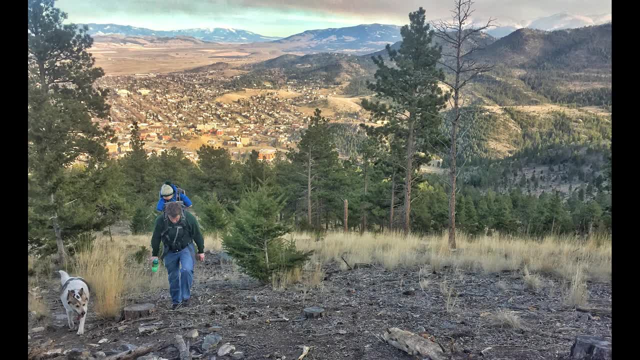 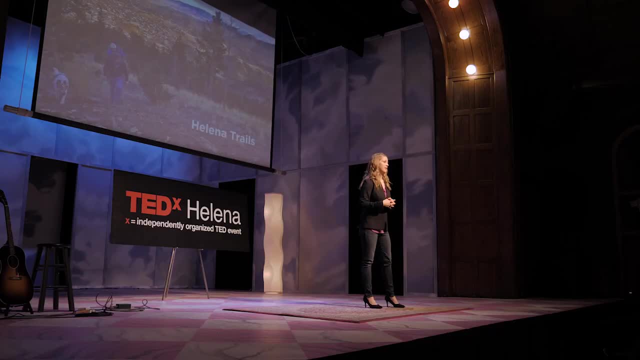 this way, and so you follow the signs and you go up there. You see a large parking lot. many times it's filled with cars, so it is being used. you can see that, And part of reading the landscape is also seeing how people interact with the landscape. 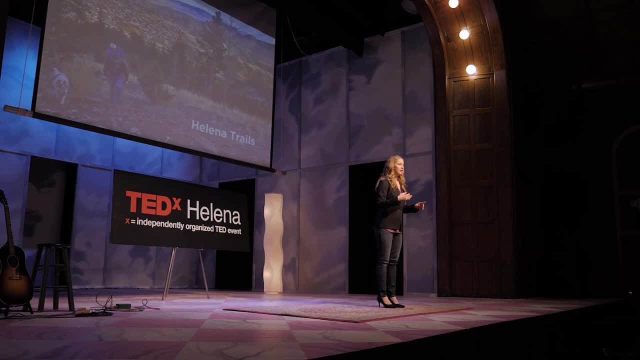 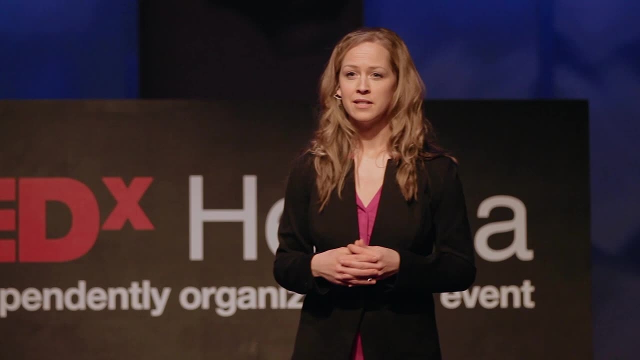 And so you go on the trails and you see the runners and the bikers, the hikers, the toddlers, the organized groups. they're all utilizing the landscape, And that's all part of this landscape and part of Helena's place identity as a community that's invested in its local trails. 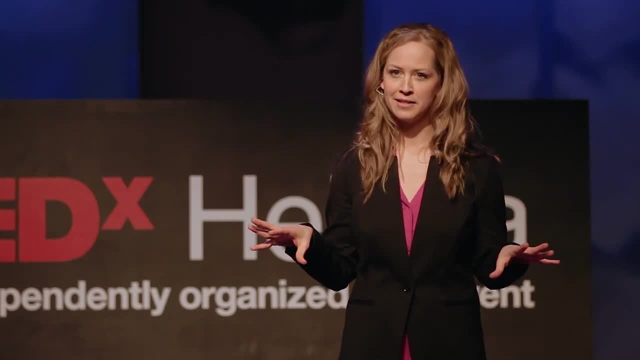 And then when you're out on the trails, be sure to look out. There's a lot of different things that you can see, But one thing to take note of is the street patterns. We see our nice straight streets, that nice grid. And there's a connection there that goes all the way back to 1682 and William Penn, when he laid out the city of Philadelphia. He wanted that grid pattern, And real estate sellers and buyers loved it too, because it made the selling of lots nice and easy and convenient. 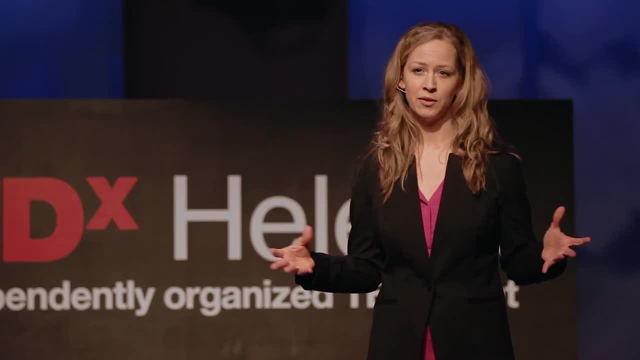 And so we're in Helena. we have our local trails, but we're also Westerners, and so we're surrounded by public lands, from national parks to national forests, And there's a couple different ways we could look at the national parks. 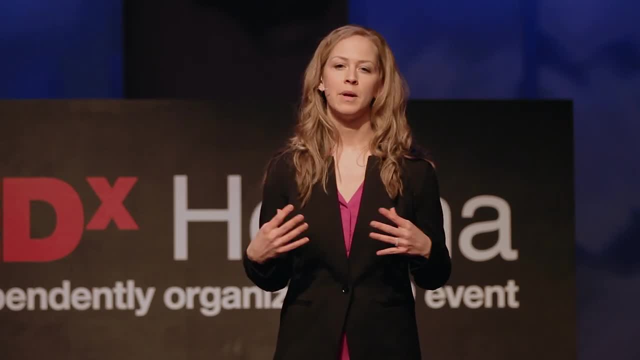 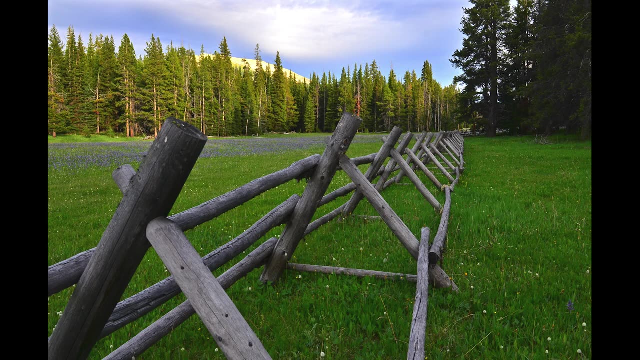 What I want to focus on is how they're managed as lands of many uses, And this isn't a new idea either. This goes back to the late 1800s, early 1900s, when much of the public stewardship of the forested mountain areas 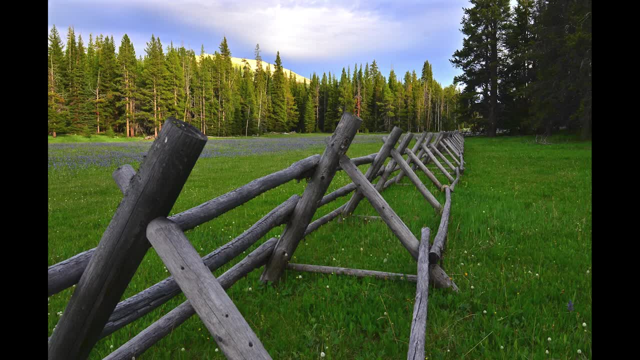 fell into place, And so we have our lands of many uses, and that's going to differ depending on which forest you're in. So in this one here, this is in Pioneer Mountains, and on one side you have your grazing allotment. 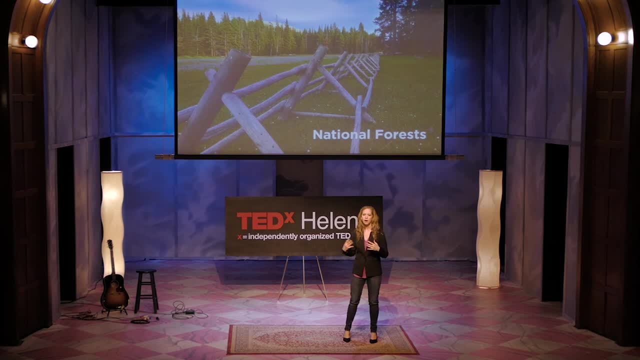 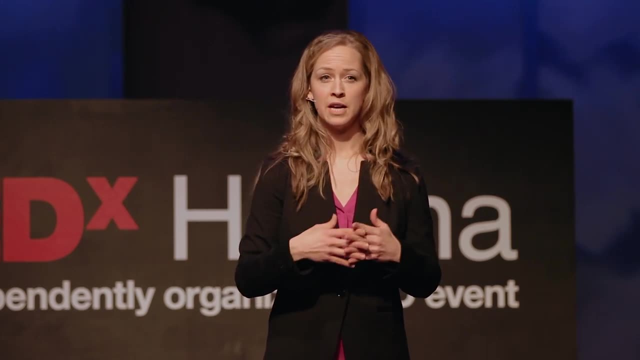 So you have cattle grazing fence separating that from the campgrounds. Others you're going to see, like commercial logging and logged areas and reseeded forest And going back to the recreation, just the trails themselves are signs for hunting regulations And so when we see these signs of many uses, 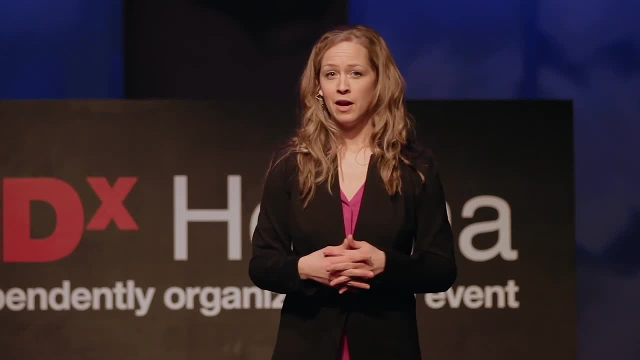 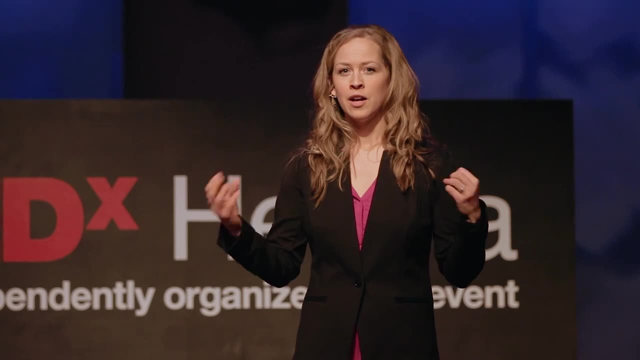 what's that saying about our culture? What do we value, whether that's economic values or cultural values, or traditions being carried on or just like what we like to do in our leisure time, especially as Westerners, and being outdoor enthusiasts- Enthusiasts is kind of part of our Western identity. 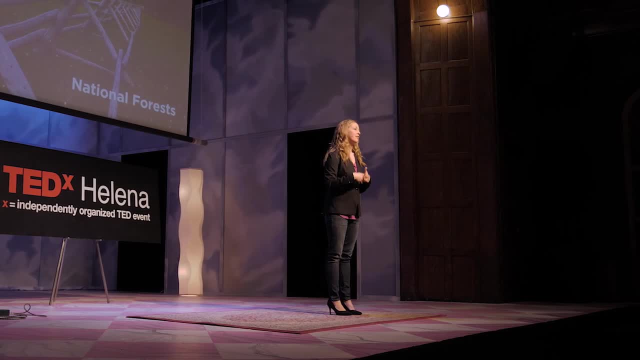 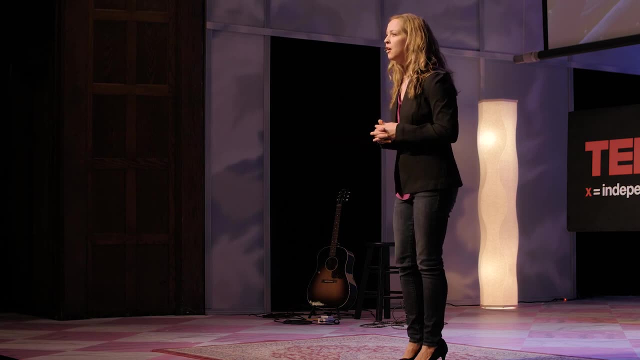 And so we have our landscape and we can read it from different scales. We can look at it from the international impact on local landscapes through such things as immigration, both the past and in the present. that's still happening today. We can also look at national policies on the landscape.